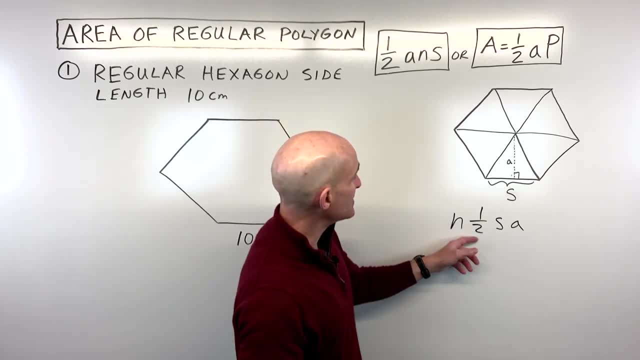 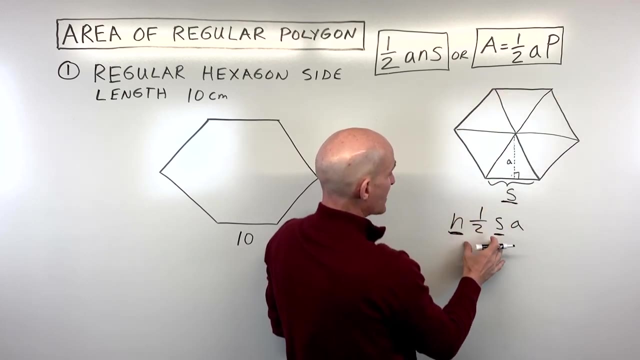 that's going to give you the area of the entire polygon. Now you can see this formula here. multiplication is commutative. you can change the order you're going to get this formula And if you recognize that the side length okay- times the number of side lengths, that's actually equal to the perimeter, And so that's. 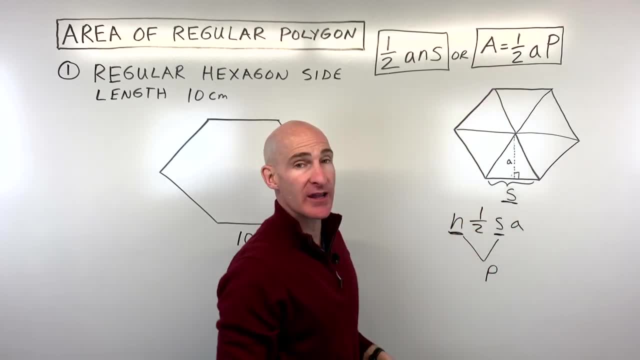 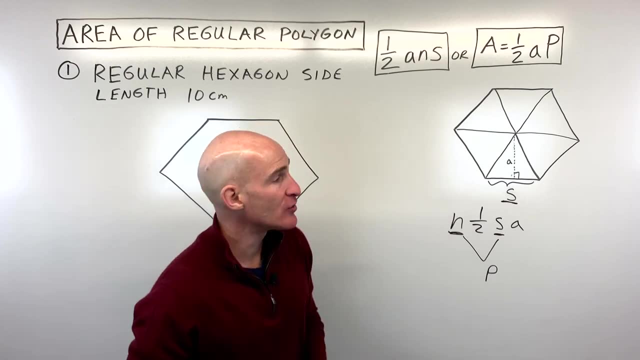 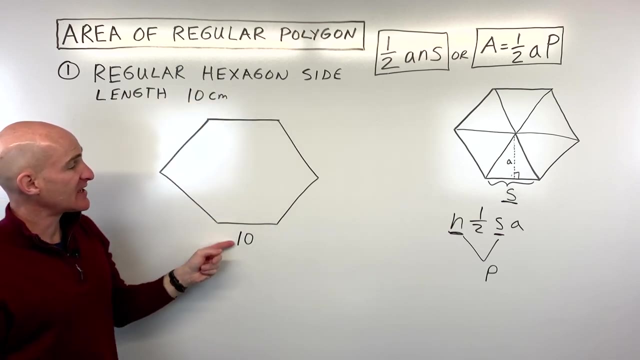 how we're getting one half apothem times perimeter, this formula right here. So again, if you ever forget, just find the area of one triangle, multiply by how many triangles you have. So let's dive into the first example, And I want to show you how to do this: A regular hexagon that has a side length of 10 centimeters. 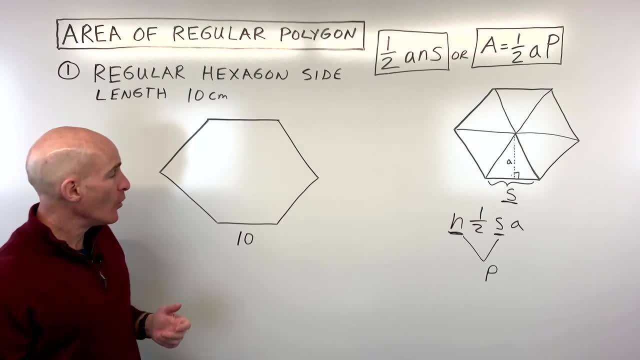 that's all we're given. How do we find the area? Well, go ahead and pause the video, see if you can do this one on your own. But if I was going to do it, what I would do is I would find the center of that polygon and I would subdivide it into triangles, like I was showing. 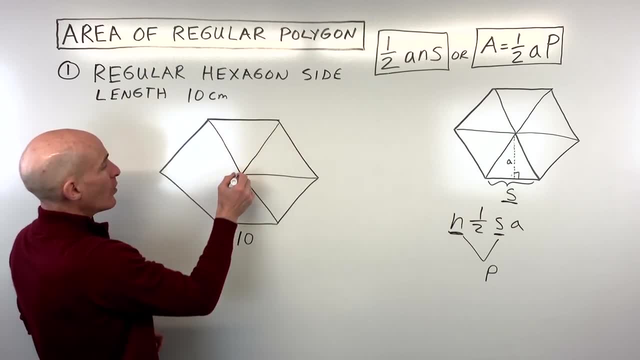 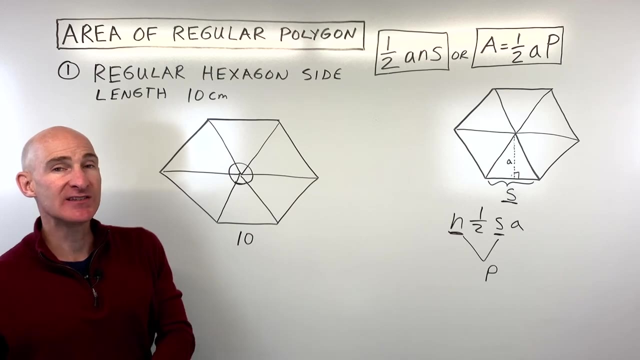 you earlier over here, And what we have here is what's called a central angle And that central angle, if you think about this, this is like a circle which is 360 degrees, But if we divide that by these six angles here at the center, 360 divided by six is 60 degrees, And so let's label 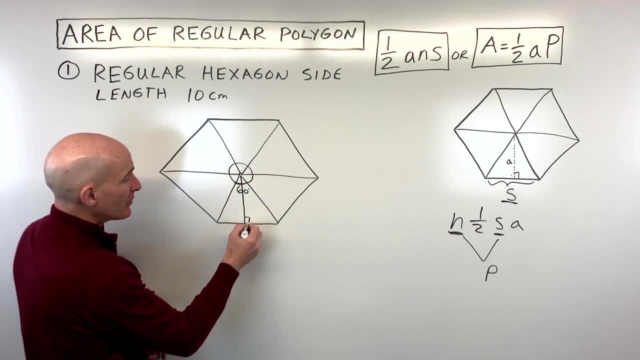 that 60. And then if we drop an altitude, okay, which represents the height of this triangle, what happens is it's going to bisect this central angle, which is going to make this a 30 degree angle for each of these triangles. And when you drop that altitude, 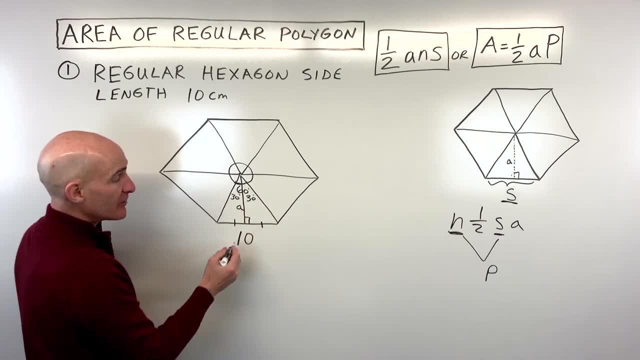 which we call the apothem. it's also going to bisect the base or cut that base in half. So each of these guys is going to be five. So let's take a look at this triangle Now. you can see it's a 30,. 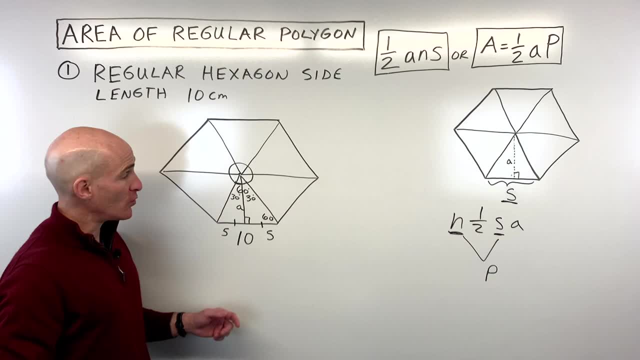 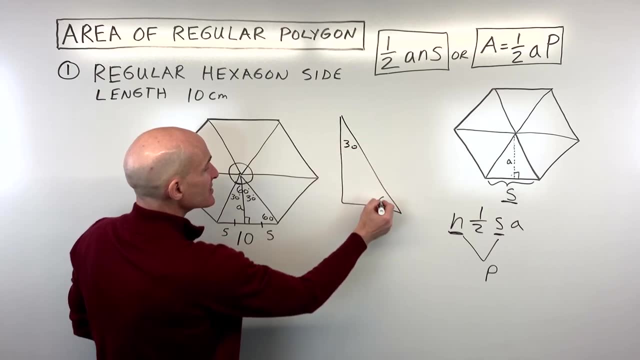 60, 90 triangle, because all the angles in a triangle add up to 180.. This is a special right triangle, So let's just draw that a little bit larger over here so we can see it: 30,, 60,, 90,. 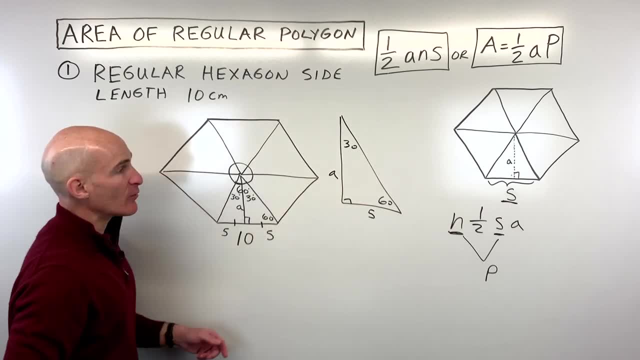 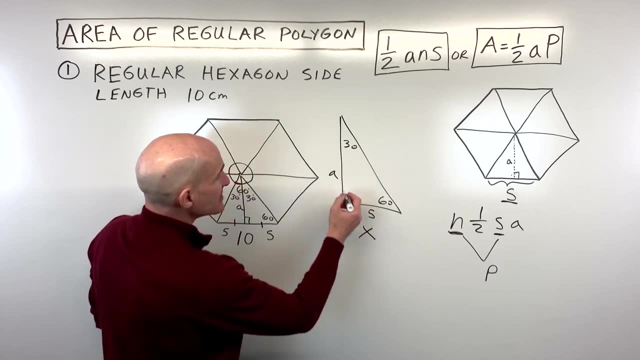 this is five And this is our apothem, And we want to figure out what this side is here. Now. you probably remember from earlier: in math this is called x. this side here is called x, square root of three and the one. 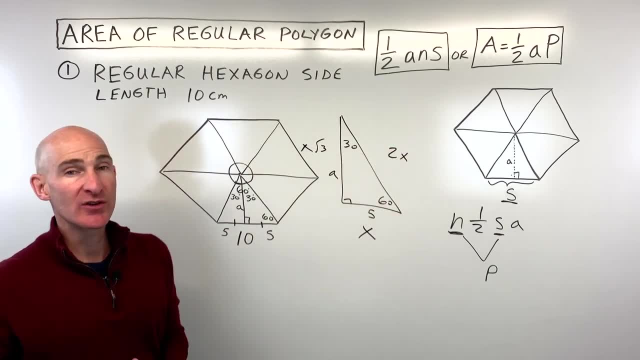 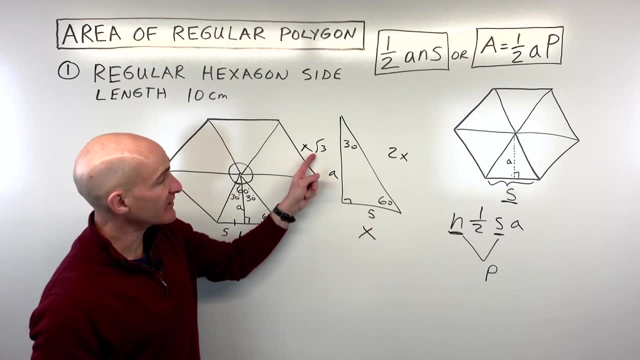 across from the right angle, that's two x. These are the ratios that we see in a 30,, 60, 90 triangle. So if we're given this side here, the short leg, five to get to this longer leg, this x root three. 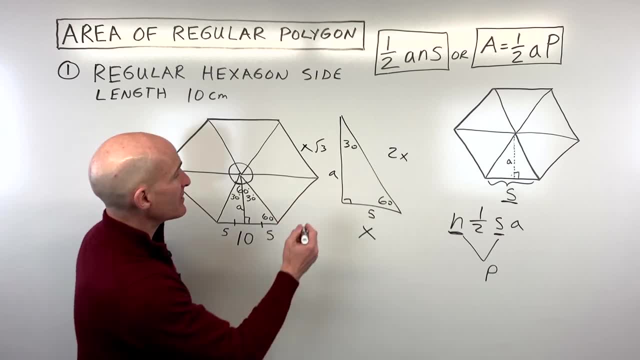 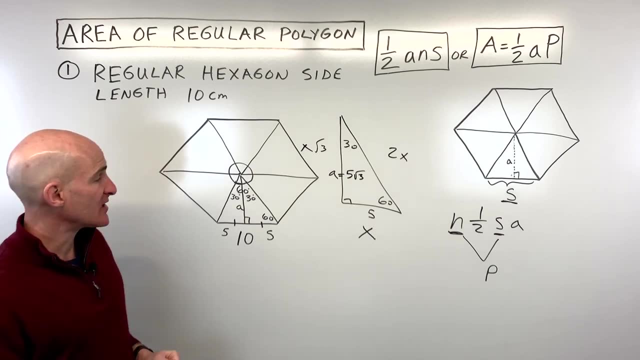 side, we have to multiply by the square root of three. So that means that a here is going to be five root three. Now I'll show you how to do this, using trigonometry and sine cosine tangent ratios, but let's just set this up first. So we're going to use this formula: one half apothem times the. 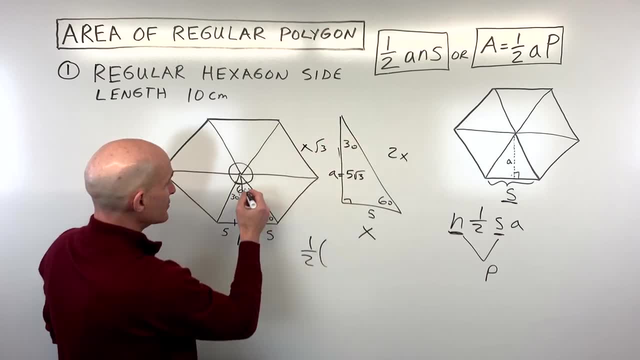 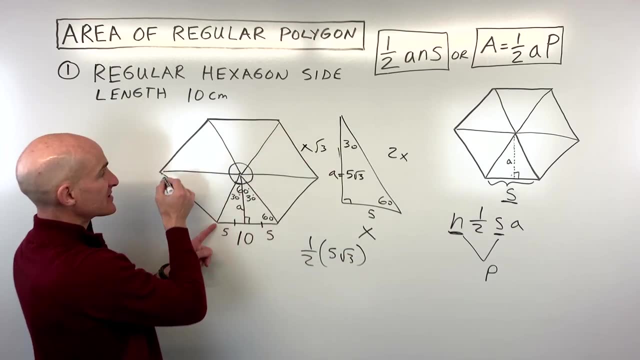 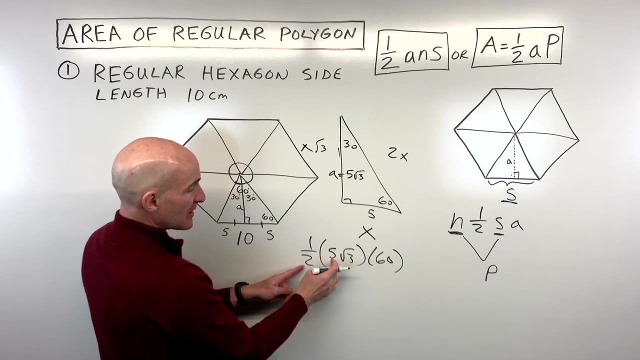 perimeter. So we have one half the apothem which is the height of this triangle right here We said it's five root three times the perimeter. Now that's going to be 10 times six sides. So that gives us a perimeter of 60. And if we multiply that together, let's see a half times 60 is 30. 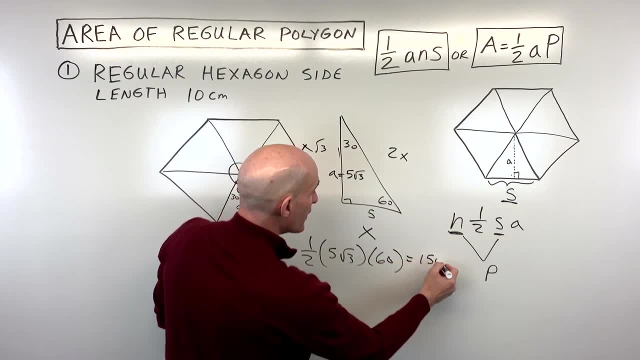 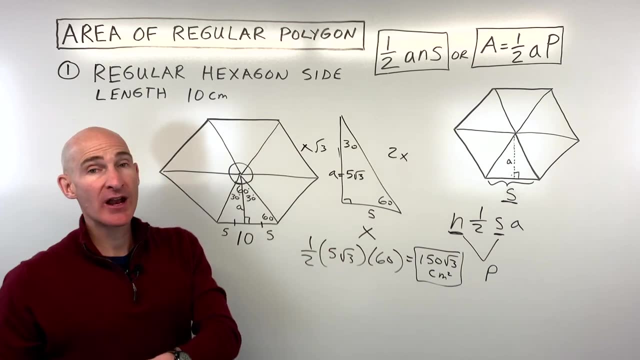 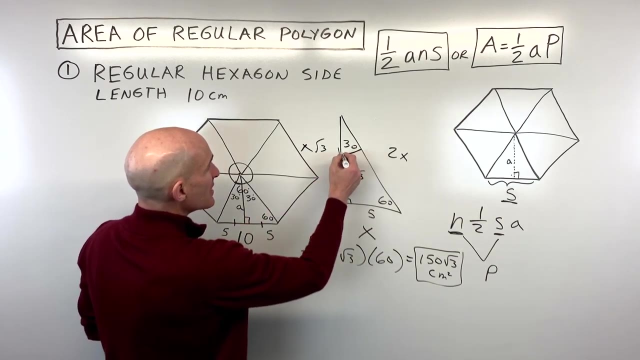 times five is 150 square root of three. So 150 square root of three centimeters squared. That's the area. Now let me show you how to do it. if you didn't know how to use the 30,, 60, 90 triangles, What you can do is you can position yourself here at this angle: 30 degrees. 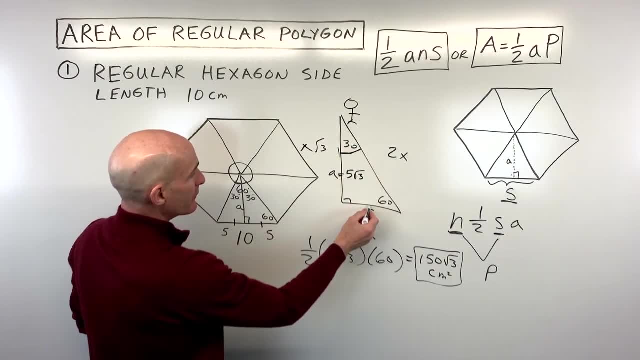 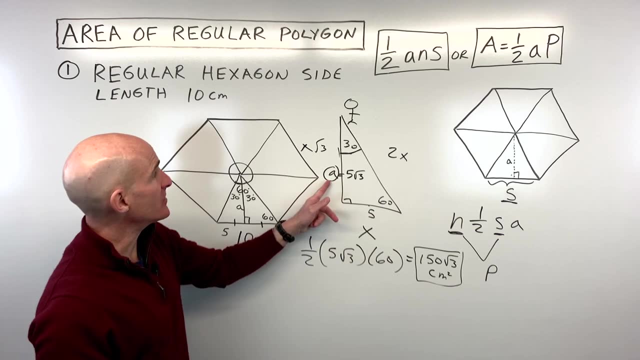 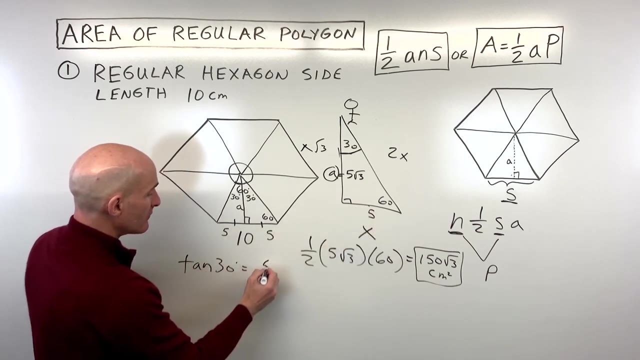 and you can say what trig function ties together the opposite side five and this adjacent side a, which let's just say we don't know. Well, let's see opposite and adjacent, that's tangent. So what we can do here is we can say the tangent of 30 degrees is equal to opposite five over adjacent. 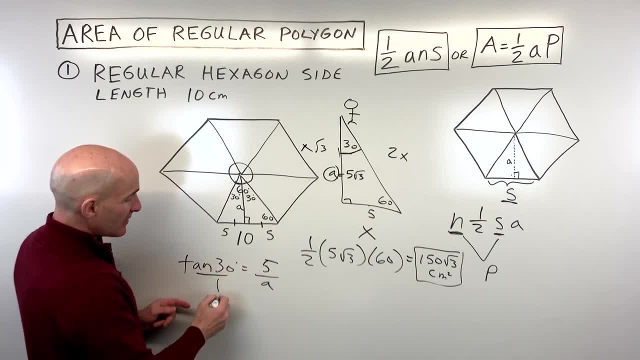 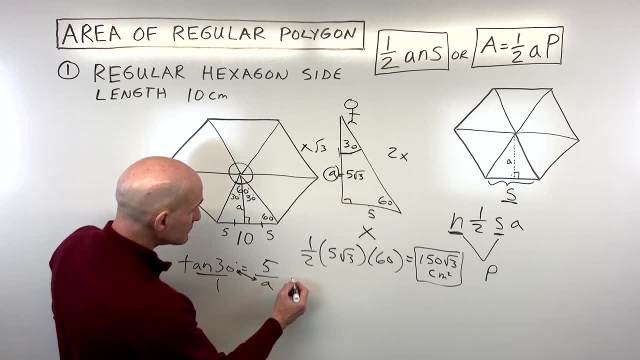 a. Now we can cross, multiply and solve, or there's a property of proportions that allows us to interchange these on the diagonal. So this would be a over one, which is: a is equal to five divided by the tangent of 30 degrees. And then what we can do, that we can. 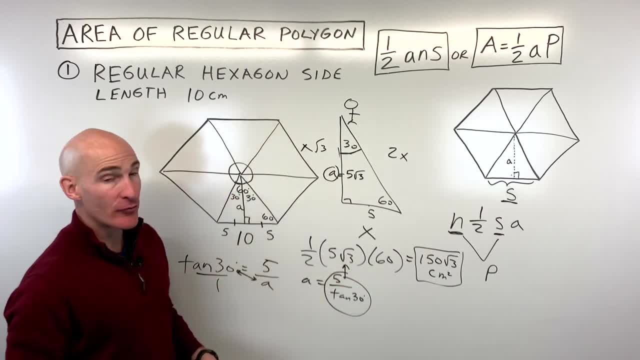 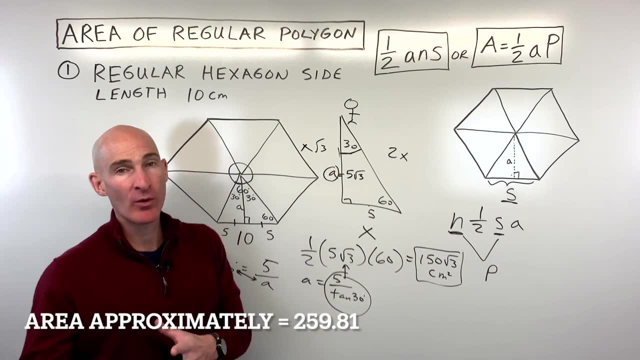 put in place of our apothem right here: five root three. The only thing is, when you do it this way, you're going to get like a decimal approximation instead of like an exact answer. So, depending on what the problem is- asking for exact answer or rounded answer- you can do it either one of those. 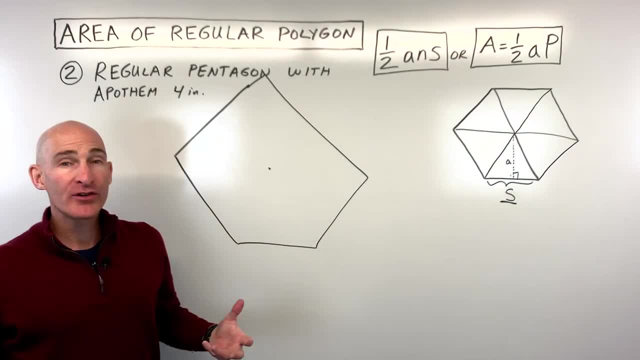 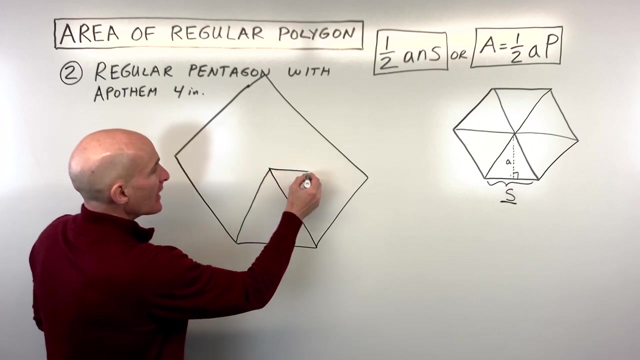 ways. So let's dive into the next example. Okay, for example number two. now see if you can do this one. It's a regular pentagon with an apothem of four inches. So let's go ahead and do the technique of dividing this up into congruent triangles, And then what we're going to do is we're going to drop. 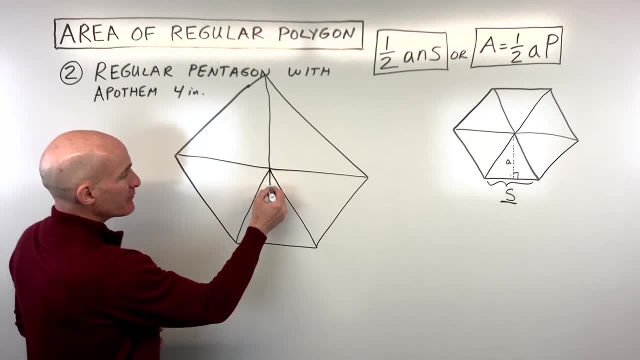 an altitude of one of these triangles. I usually like to do this one at the bottom, And that's what's called the apothem Right here. so this is a is equal to four inches. Okay, so now what we're going to do is we need to. 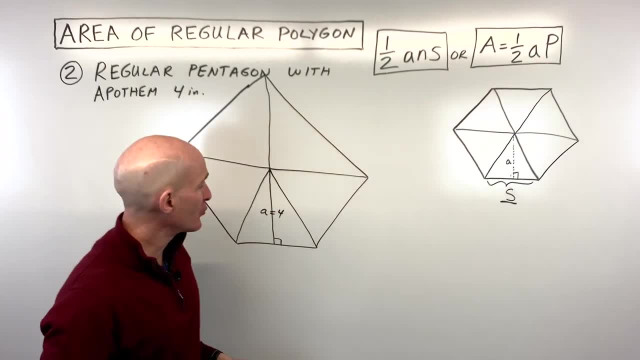 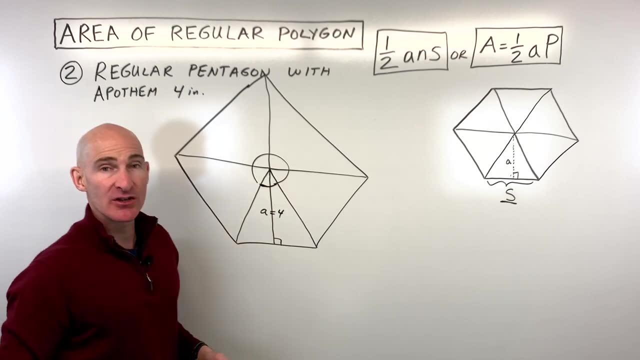 figure out what the perimeter is. We have the apothem, but we don't have the perimeter. So first thing I like to do is figure out what is this central angle? here Again, we said this is a circle, 360 degrees, but you can see that we have five triangles. So 360 divided by five is 72. 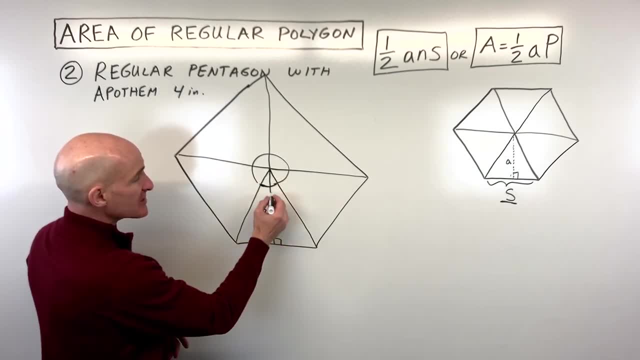 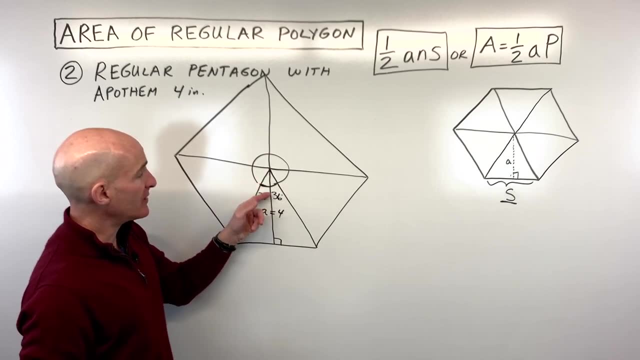 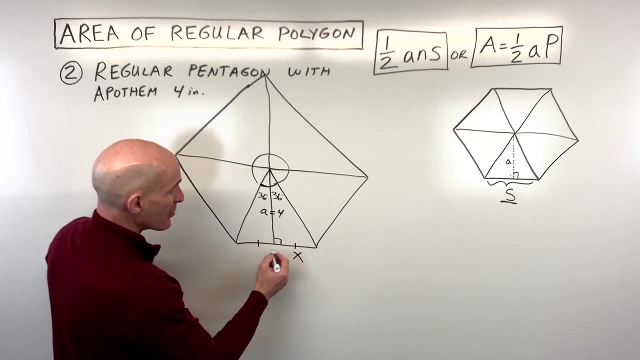 degrees. But then when we drop that altitude, half of 72 is going to give us 36 degrees. So that's the key is to find that central angle and then cut it in half. Now, when we do that, it's going to bisect the base and let's just call this length, just this part here, x and this part over. 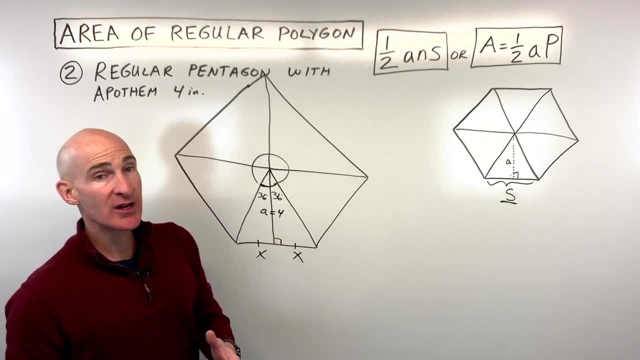 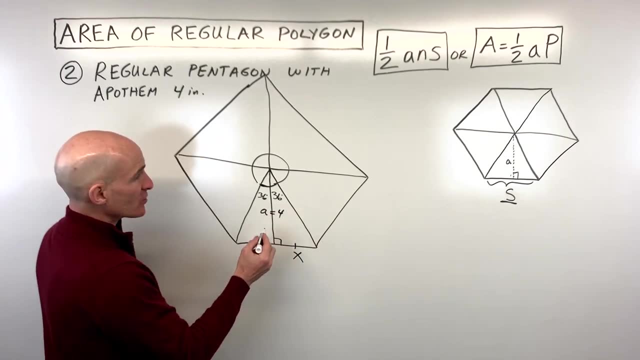 here x. So here what we have to do is a little bit of trigonometry to find out what this piece is here. So we're going to say opposite and adjacent is tangent. So we're going to say the tangent of 36 degrees is equal to the opposite side, x. 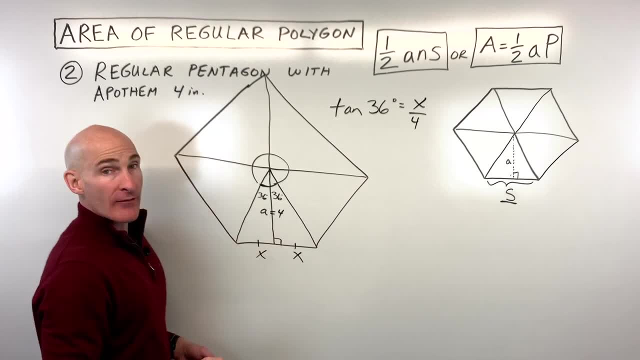 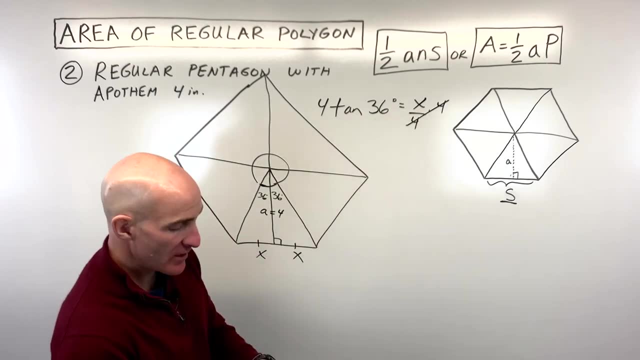 Over the adjacent side, four. Now all we have to do is multiply both sides by four to get x by itself. So let's go to the calculator. on that one, Make sure you're in degrees. and four tangent 36 comes out to about 2.906.. Okay, we'll just carry it out a little bit. so 2.906.. 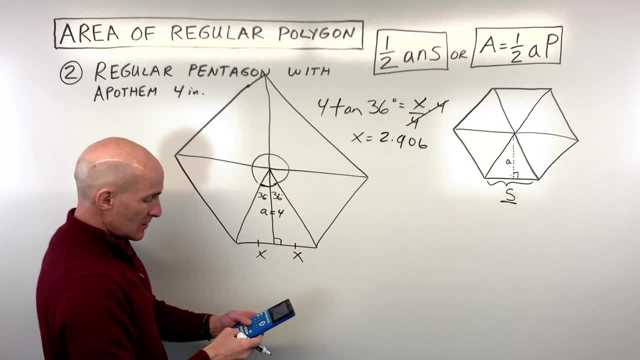 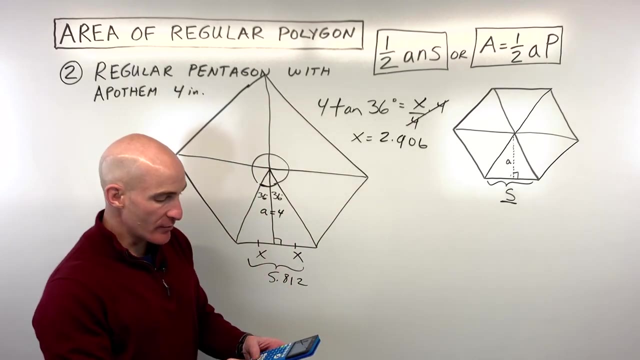 And what I'm going to do now is I'm going to double that to get the length of one of the sides. So if I multiply this by two, this is actually going to come out to 5.812. and then if I multiply it by five sides, that's going to give us the perimeter. So let's multiply that by. 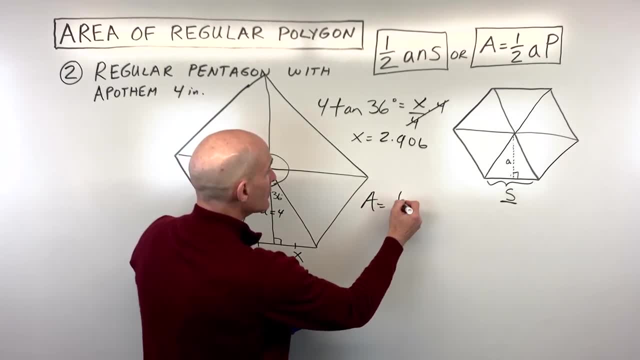 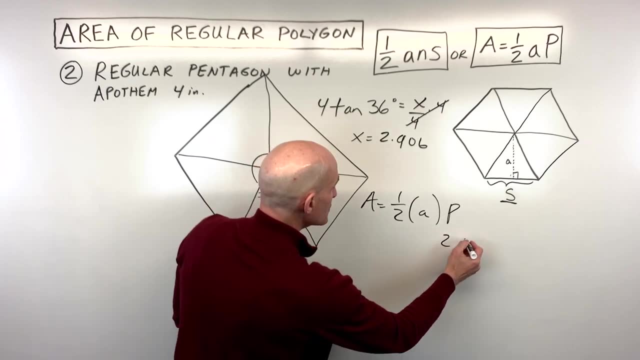 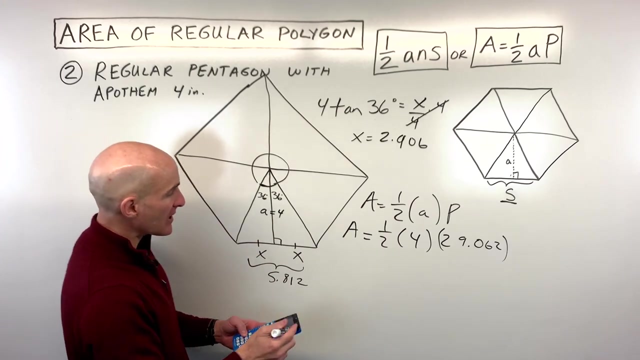 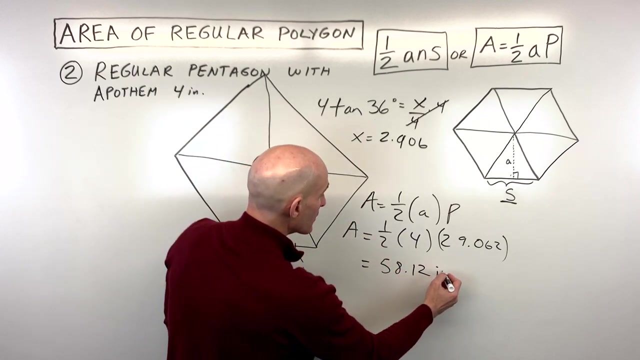 five. So it looks like our perimeter now is going to be, let's see, 29.062.. So 29.062, we've got our apothem, which we said was four. And if we multiply all that together- let's see times 0.5 times four- we should be getting approximately an area of 58.12 inches squared. 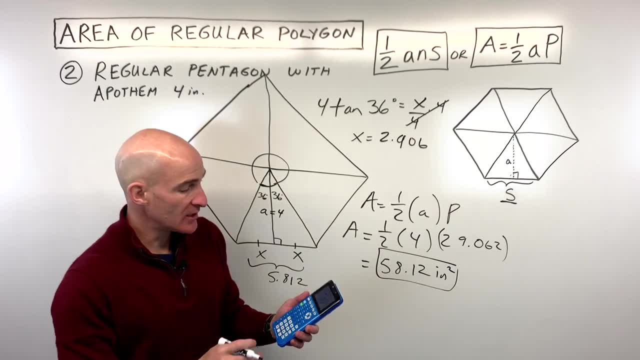 And that's your area. now. What I try to do when I do these problems- just a little hint- is I like to kind of carry forward those numbers, So if you can use the previous answer key and carry forward that long decimal, and I try to save rounding for the very end. 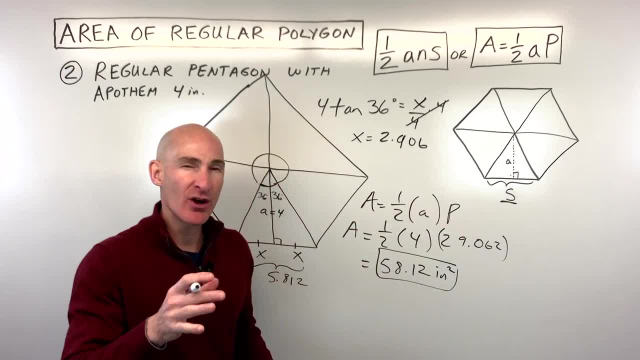 to get a little bit more accurate. If you keep rounding each time you'll be off a little bit. It's like a rounding error and you keep rounding, rounding like that, It throws you a little bit off. So try to carry as much of that decimal forward. 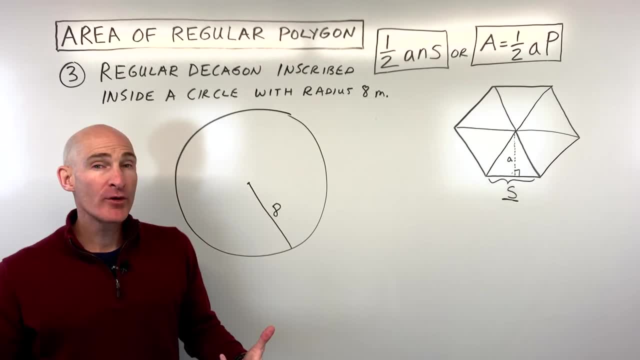 Let's take a look at example number three. Okay, before we dive into example number three, if you enjoy my content here on YouTube and you find yourself coming back to my videos now and again, consider supporting the channel by joining as a channel member. 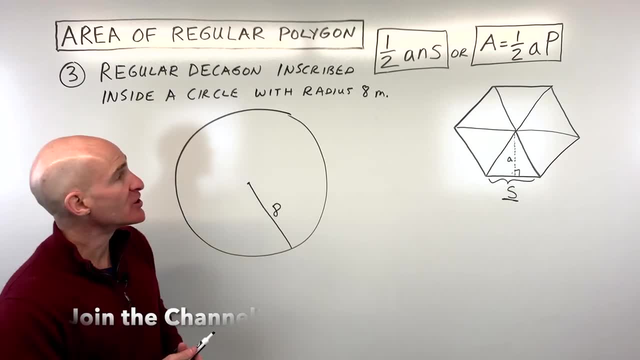 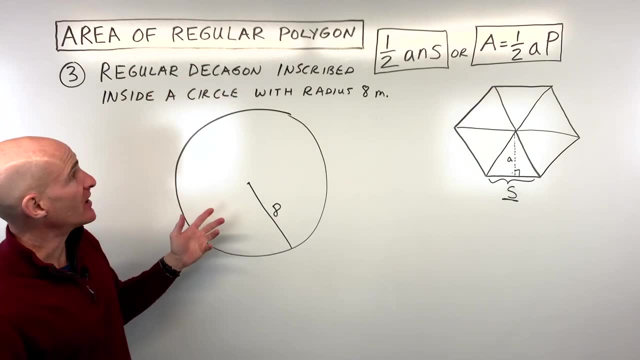 It really helps me out and I appreciate it. So let's jump into example number three here. Basically, what we're given is a regular decagon, which means it has 10 sides right And it's inscribed inside a circle with radius eight meters. 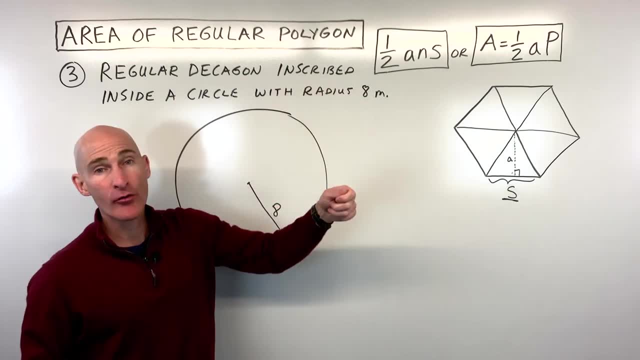 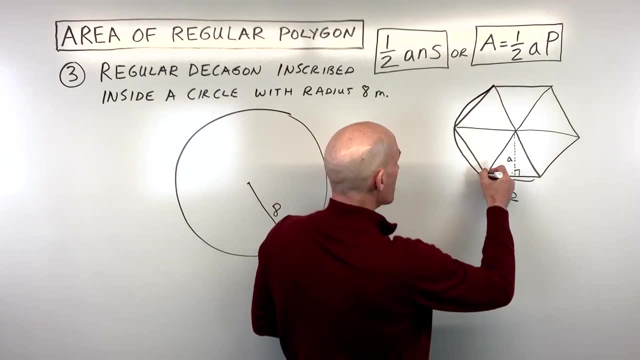 Now, what does this mean? inscribed? Well, scribe means to draw or write, and it's on the inside, And you can think about this as the circle is being circumscribed or drawn around the polygon, like this, And so when we talk about the radius, 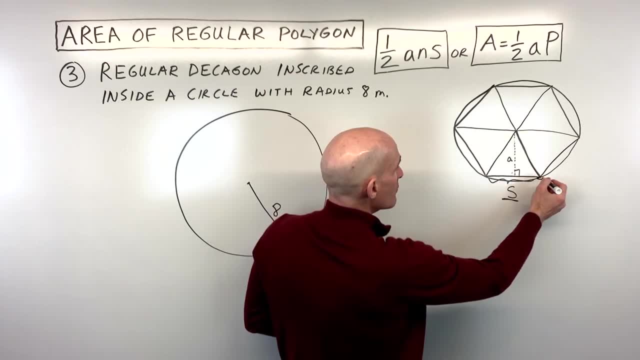 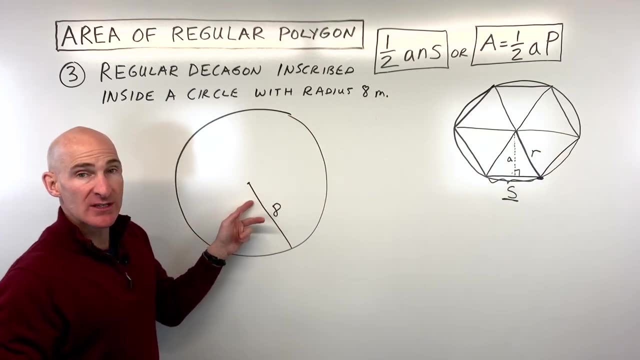 we're really talking about this dimension right here, from the center to a point on the circle. So this is our central angle, or a vertex of the polygon. So this is our radius R right there. So here, what I'm gonna do is I'm gonna just draw. 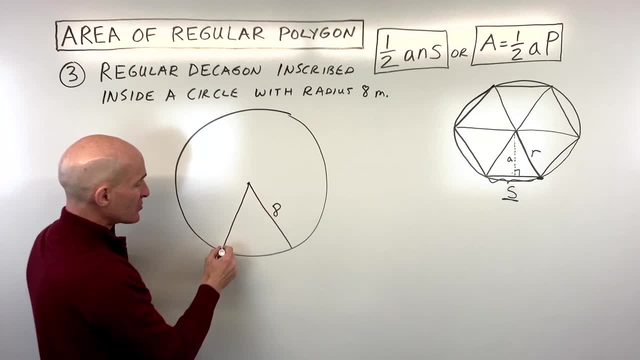 one of these triangles of our decagon. So if I was to kind of illustrate like this: say this is just one of the triangles, imagine you had 10 of them. okay, all the way around this. okay, continuing like that. 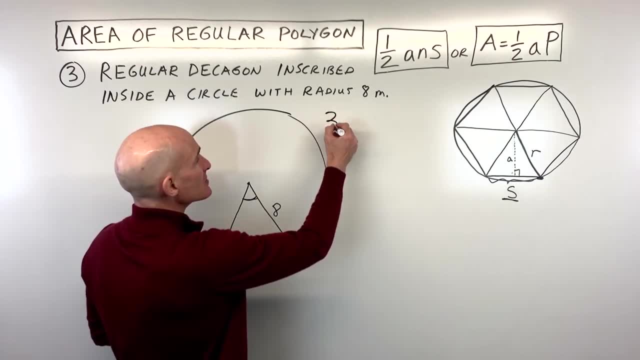 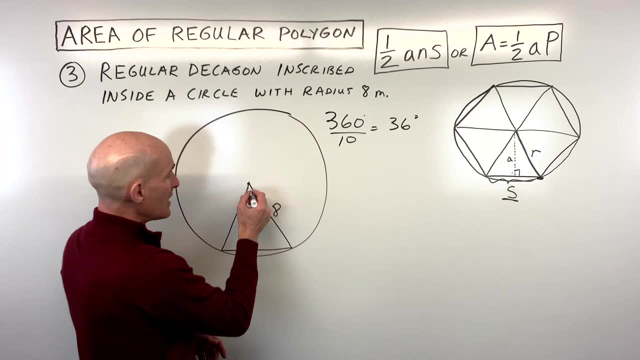 We need to find out what the central angle is. So what we're gonna do is we're gonna take 360 degrees divided by 10, okay, and then we're gonna cut it to a central angle of 36 degrees. Now we're gonna drop an altitude, okay. 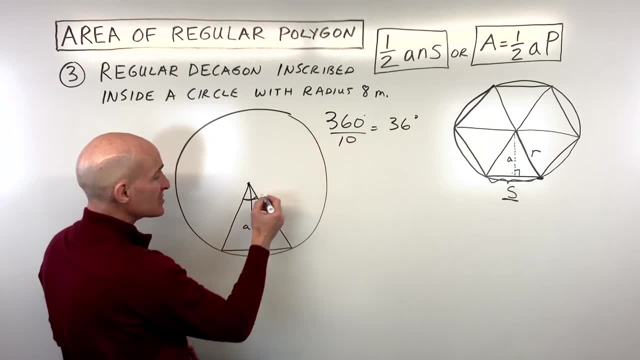 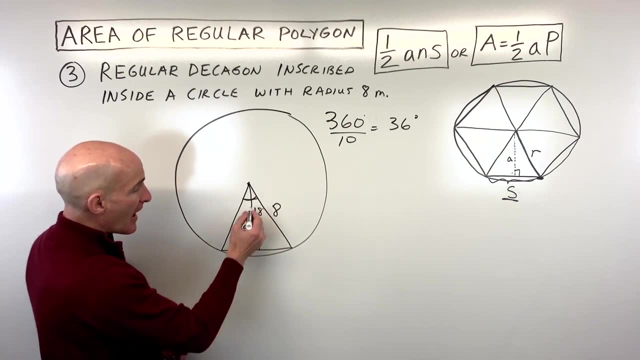 which, remember, we call that the apothem, and that's gonna bisect this central angle of 36 degrees. cutting it in half, that's 18 degrees. Now what we need to do is we need to figure out what the apothem is. 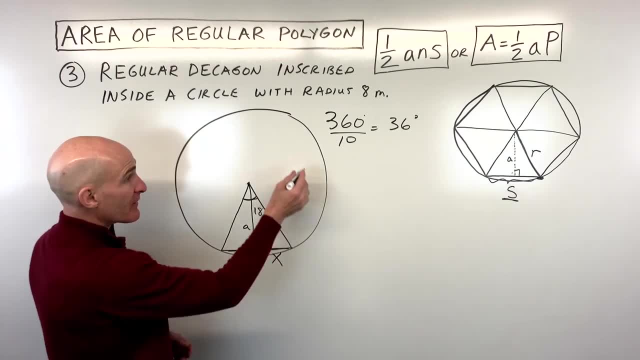 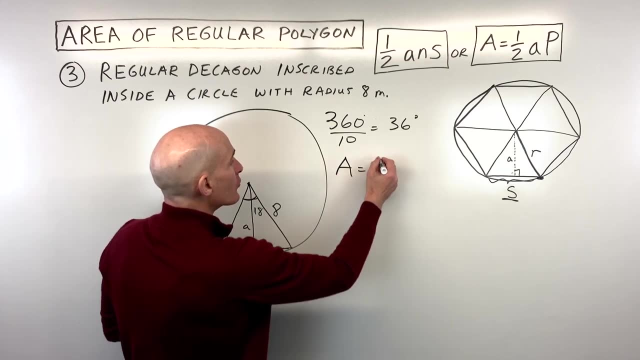 We also need to find out what this side length is here, so that we can find the perimeter. So let's start off by finding the apothem. Now, one thing I like to do sometimes when I'm doing these problems is, you know, 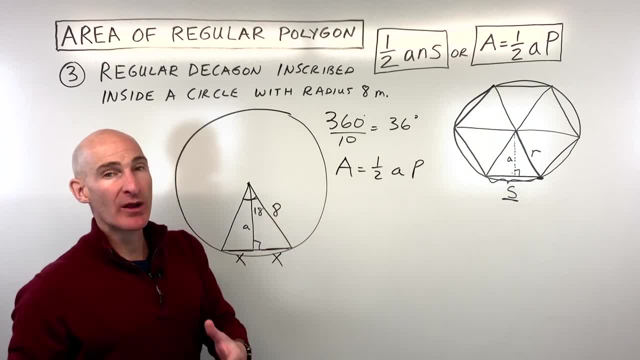 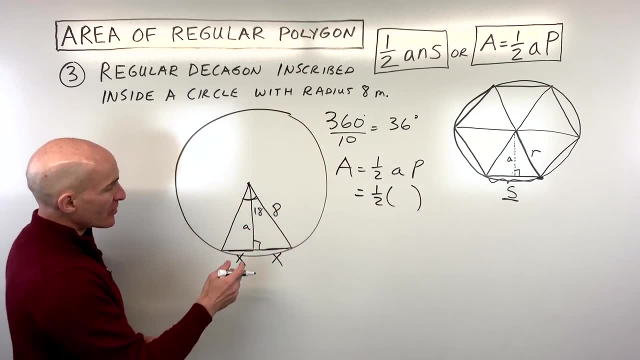 I take a formula and then kind of substitute in what I know, so I can kind of see what I'm still missing, what I need to go and find. So in this case let's go after the apothem first, And what I'm gonna do here is I'm gonna go ahead. 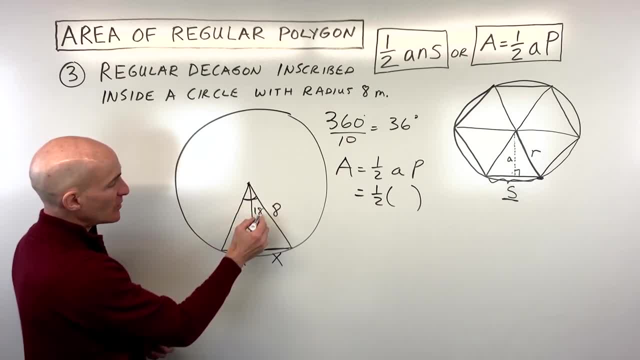 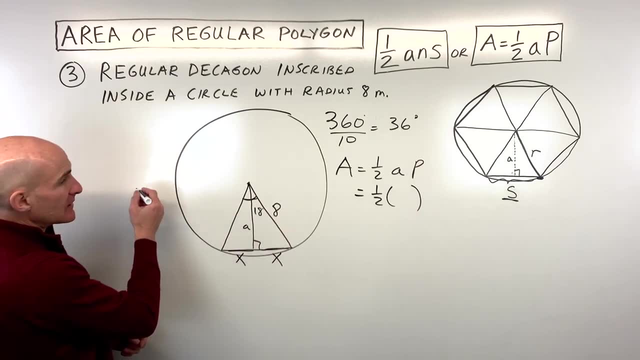 and use some trigonometry. So if we're here at this angle- 18 degrees- we need the adjacent and the hypotenuse. that's our cosine right. So let's write that down. We've got the cosine of 18 degrees. 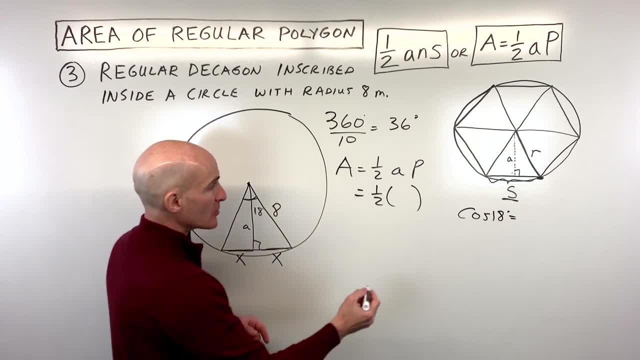 is equal to adjacent, which is a over 18, over hypotenuse eight. If we multiply both sides by eight, we can get that apothem by itself. So here I think what I'm gonna do is let's go ahead. 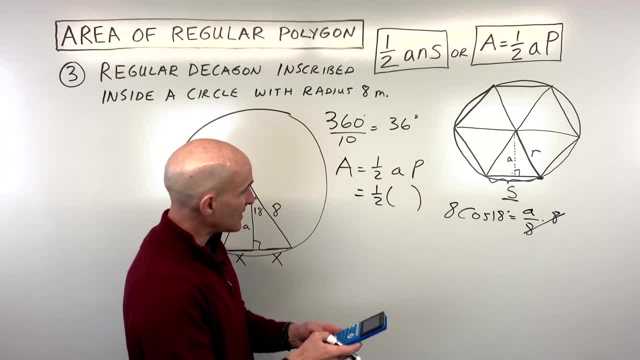 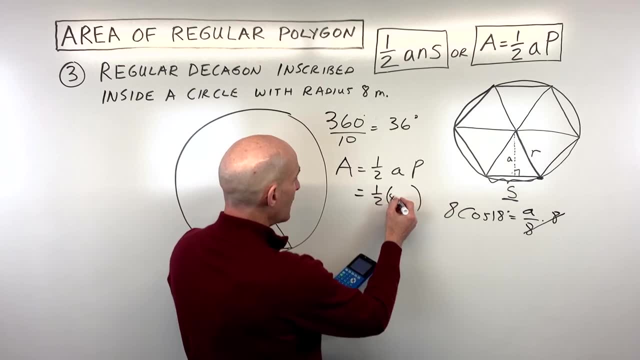 and get a decimal approximation. This is eight cosine 18,, okay, which is about 7.61,. or I'm just gonna actually write in here eight cosine 18, and we'll multiply it at the very end. This way we'll get a little bit more accurate, okay. 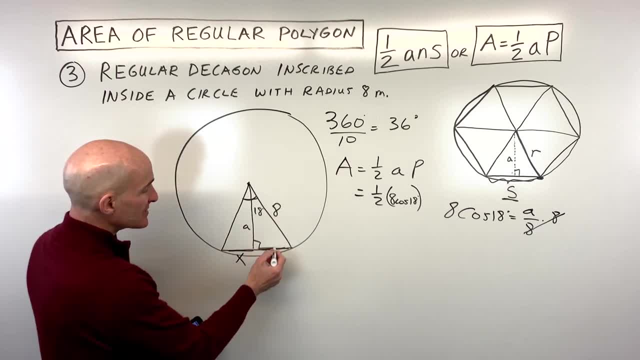 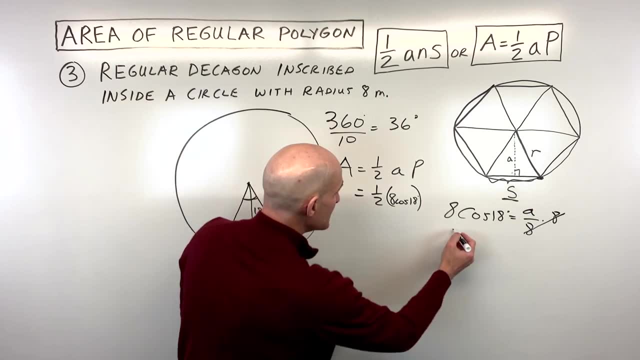 And then for the perimeter, let's go ahead and figure out what this side is. here We're gonna use the opposite and the hypotenuse, which is our sine. So we're gonna say that the sine of 18 is equal to x over eight. 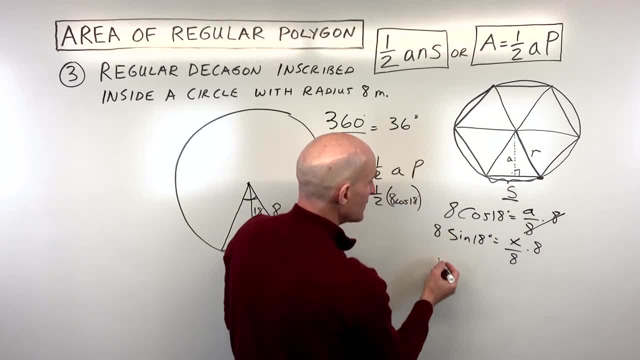 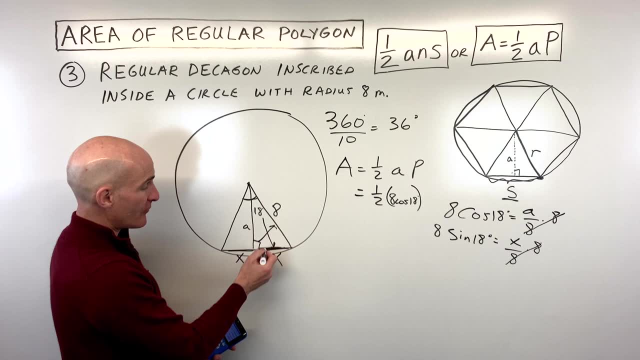 So opposite over hypotenuse Here. if we multiply both sides by eight, you can see that's gonna give us x, but then we're gonna have to double it, right Cause we have, you know, this is just half of one side length. 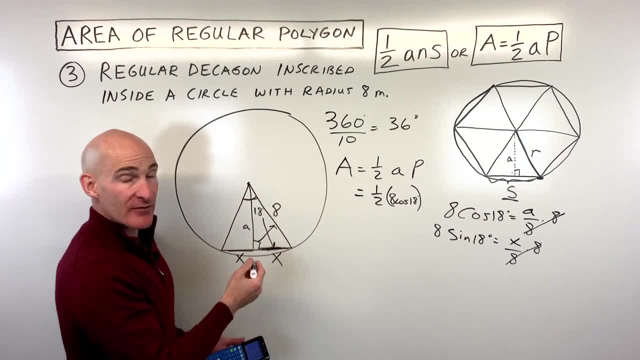 So we're gonna double it And we're also gonna have to multiply it by 10, cause we have 10 side lengths. So it's really really easy. It's really like multiplying by two and then multiply 10.. That's like multiplying by 20.. 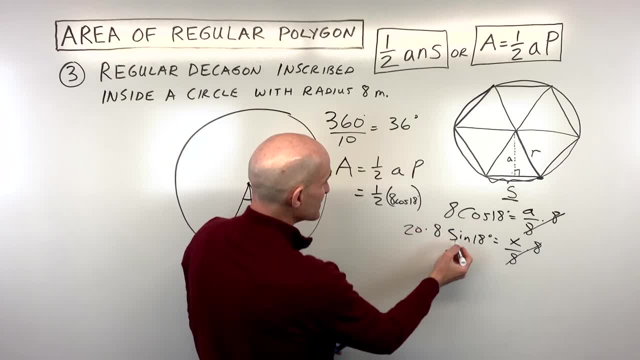 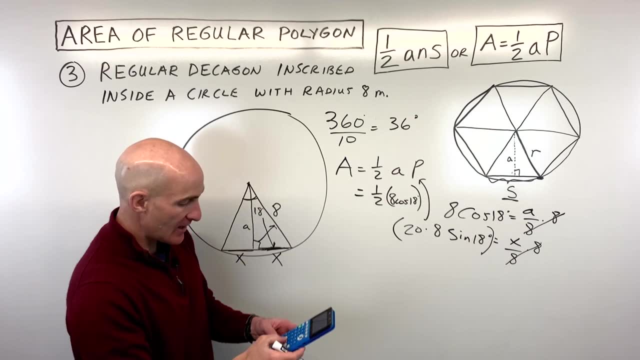 So this is really gonna be 20 times eight sine 18.. And that's gonna be what our perimeter is. So if we multiply all that together now, let's see we've got 0.5, which is a half times eight cosine 18.. 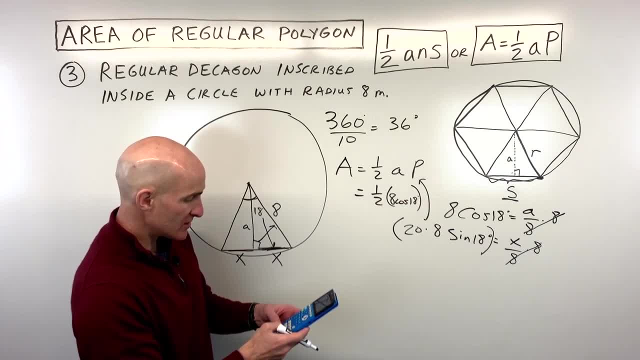 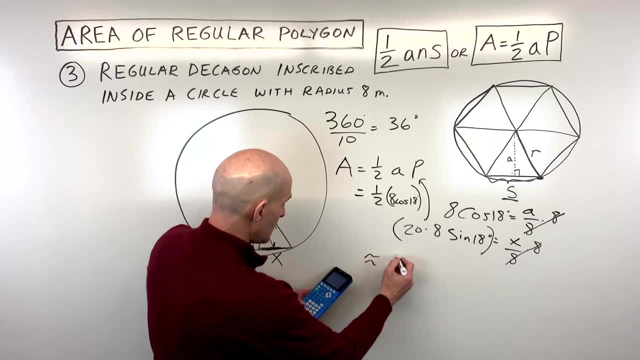 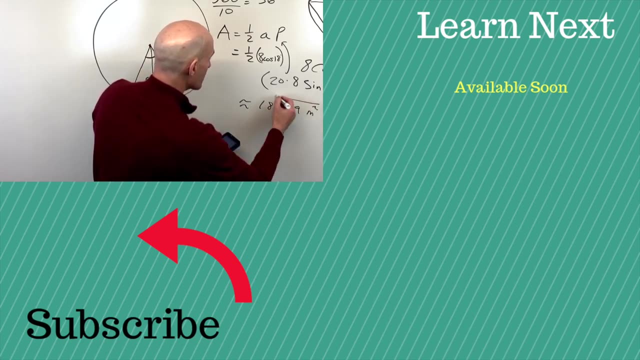 Let's see: times: 20 times eight is 160 sine of 18. And it looks like we're getting now approximately 188.09 meters squared. So that's the area of this regular decagon. If you wanna see some more examples, 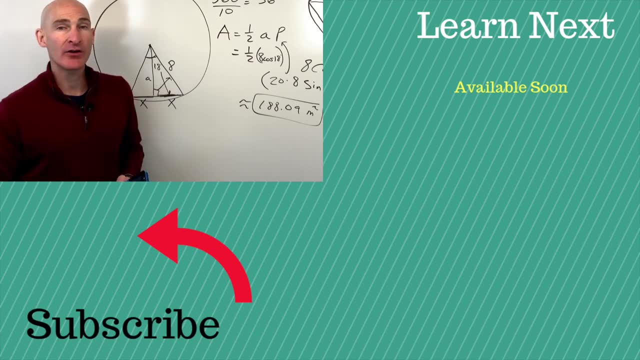 I'll put a video right there where I talk more about finding out the area of regular polygons. Follow me over there and we'll get some more practice.